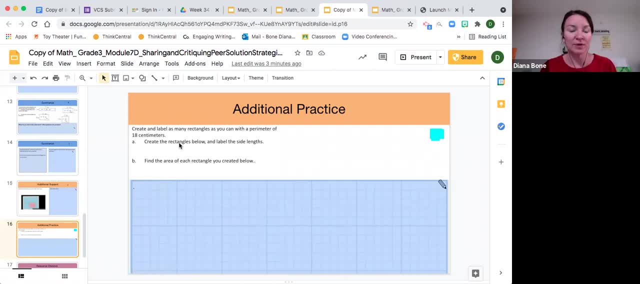 The rectangles below And we're going to label those side lengths. So, probably using- not probably using- the scribble tool. OK, so if I need a rectangle with a perimeter of 18.. On other lessons we might have started to notice that because rectangles have two pairs of equal sides, 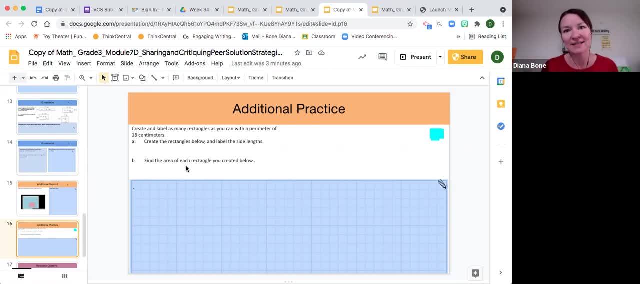 as long as two of the sides equal half of 18, the side length is going to be the same, So we're going to label those side lengths. This might be like: OK, wait a second, but you'll see what I mean. As long as two of the sides equal. 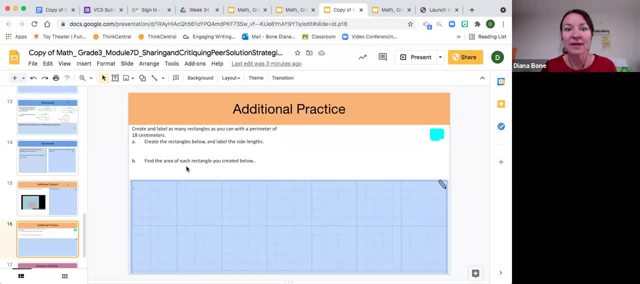 half of 18.. Your perimeter is going to be 18.. So let me show you. OK, we'll try, We'll practice. Now, not only did I say we're going to practice perimeter, but I'm going to show you how to easily. 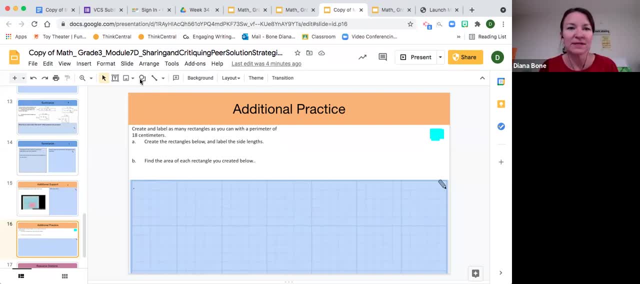 make these rectangles. Do you see up top of this little slide where you see these like beautiful little shapes, a circle and like a square behind it? It's a really cool tool To just draw a shape, like you. What do I mean? Not draw a shape like, insert a shape You don't even. 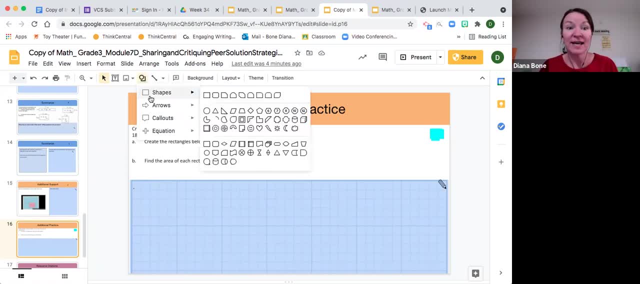 have to draw the shape. It actually, if you click on it, it has the shapes, for you See all those cool shapes, Oh my goodness. So I see a rectangle right here. So I'm going to click that rectangle and I see my little plus that tells me that's going to be the vertex, One of the vertexes- vertices. 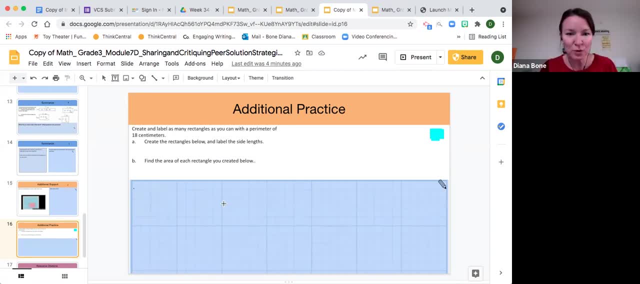 One of the vertices of the rectangle. So I'm going to make sure to line that little crisscross up on one of the squares and I'm just going to click and start dragging, Do you see? Do you see? Do you see my rectangle coming to life? I could bring it all over the 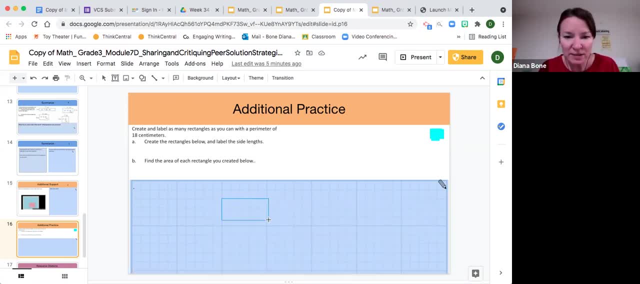 place. Now I know this would be way more than 18.. So let me bring it back and let me do that rectangle. Boom, There's a rectangle for you. You didn't even have to go line, line, line, line, It's already. 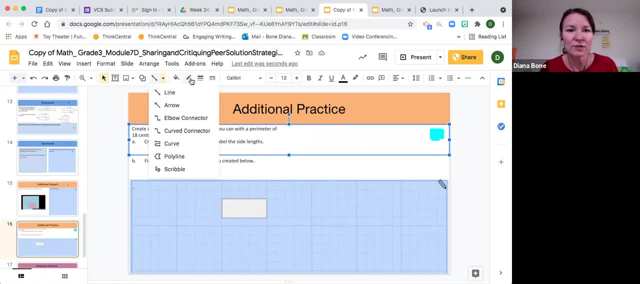 done And now we're going to use the scribble tool To sort of count, put a little check as we count the outside units, because that's what perimeter is all around the outside. So one, Two, Three, Four, Five. 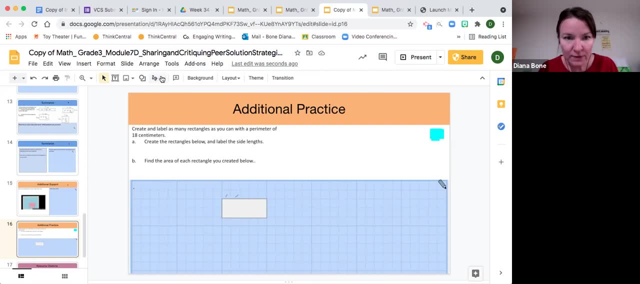 Six, Seven, Eight, Nine, Ten, Eleven, Twelve, Thirteen, Thirteen, Fifteen, Fifteen, And we're going to go around the sides Four, One And two, So let's label those and see if that works. 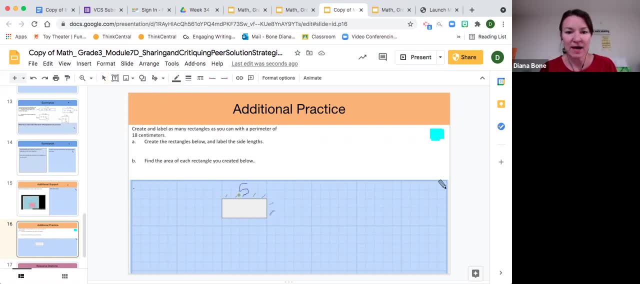 So one of my sides is five, The other side is two. let me, if one, if the top is five, the bottom is going to be five. if the right is two, the left is going to be two right. so let me add it all together, and we should know how to do that by now. 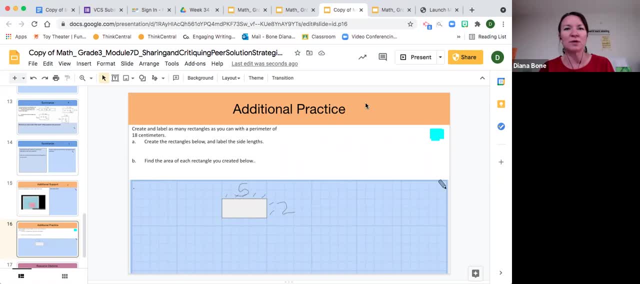 five plus five is 10 plus two is 12 plus two more. this perimeter is only 14. yikes, this actually did not work. this perimeter it's only 14. what do i do now? remember what i was saying, boys and girls that i said you might be like: this is crazy. i don't know what she's saying. we could be here all day just trying. 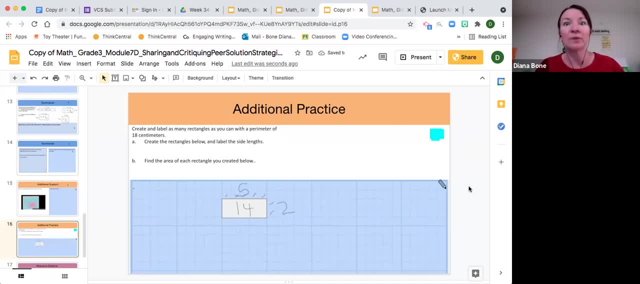 to draw a bunch of rectangles that equaled a perimeter of 18, couldn't we? we could be here all day and we could just draw a bunch of rectangles that equaled a perimeter of 18, couldn't we? we could keep counting and going: okay, that doesn't work. That doesn't work. However, if we know that two of 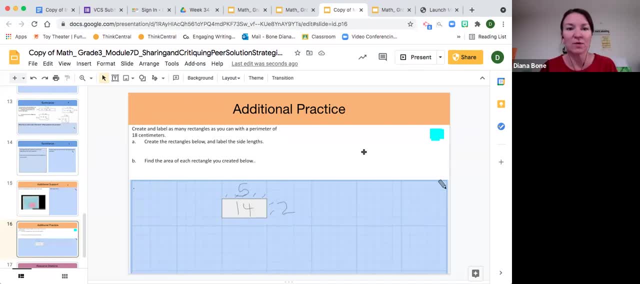 the sides are going to be equal and the other two sides are going to be equal, then really we just need to make sure that two of our sides equals half of 18.. Half of 18 is- that's right- nine. Half of 18 is nine. So it's so much easier than to think of how to make four sides equal 18.. 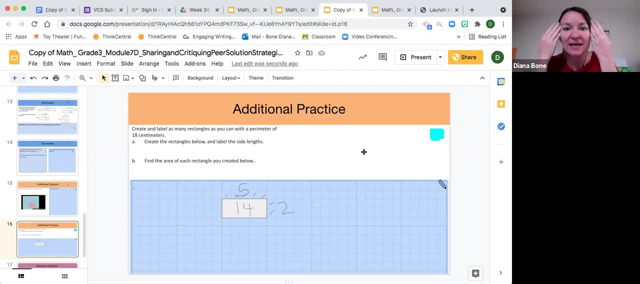 Why don't I just think about making two sides equal nine? So now we're going to get rid of this rectangle because it does not work, And then we're going to try to do that sort of thought process where we just think of two sides. 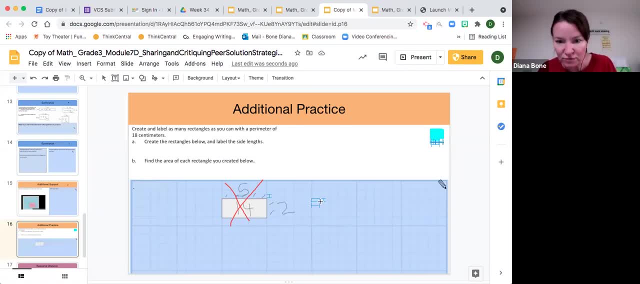 So let's start again on our vertex and let's make another rectangle. We go one, two, three, four. Let's do five across. And now what would the other side have to equal in order for both of them to equal nine? If I'm going five across, in order to equal nine I have to go one, two, three, four. 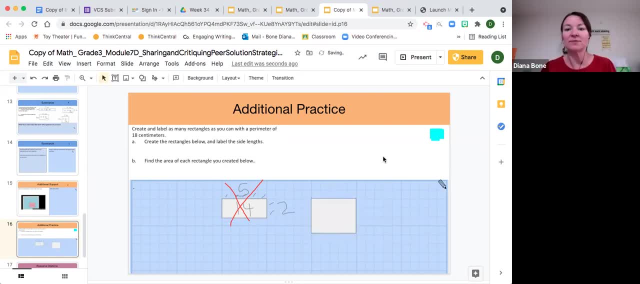 down. There you go. Now let's use our scribble tool and let's count across One, two, three, four, five. So the top side is going to equal five. And now let's go over here, get ready to write again and let's count. 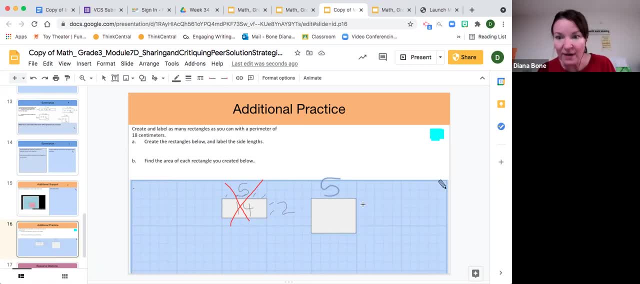 One, two, three, four. The right side is going to be four, Which means that this other side, the bottom side. well, let's reverse: What's five plus four, Nine. So the bottom side is also going to be five And the left side is also going to be four. 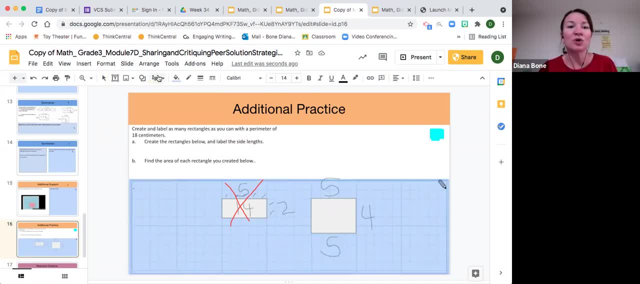 And if we thought about it, by just making two sides equal nine, it's so much easier for me than to be trying to construct these rectangles going 18 across. I'm just going to think of two of the sides. How can I make two of the sides equal nine? Now think about 18 all the way around. And now let's